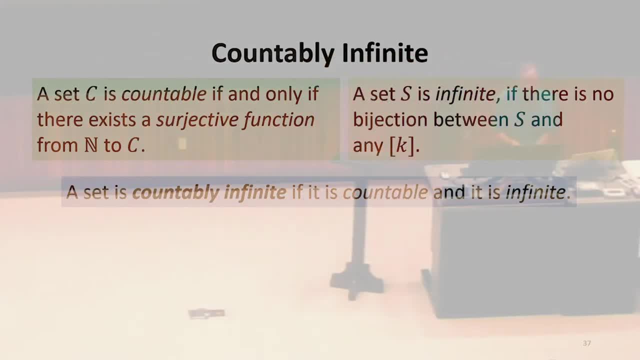 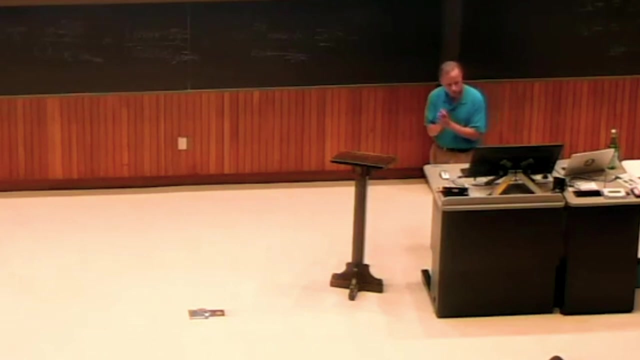 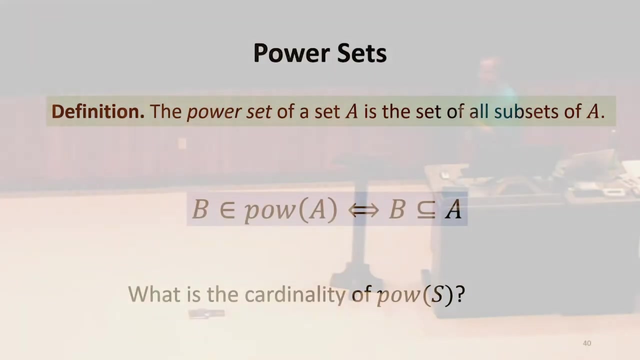 Is the binary strings countably infinite? Yeah, we know it's infinite. We know it's countable, It's countably infinite. Are there any sets that are bigger? We're going to first define the power set. I think most of you have seen this in discrete math. So the power set is the set of all subsets. 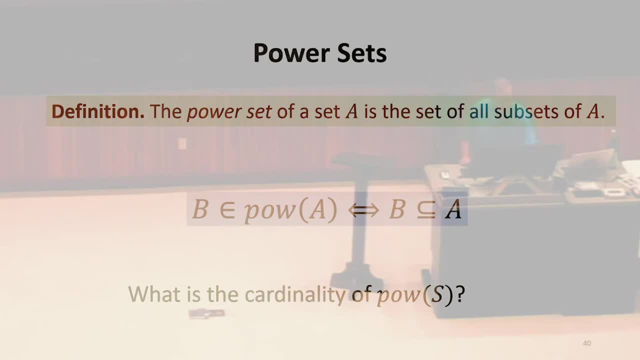 of a given set. If we want the power set of 1,, 2,, 3,, how many elements will be in its power set? Yeah, eight. So that's where the name power set comes from. It's going to have the empty set. 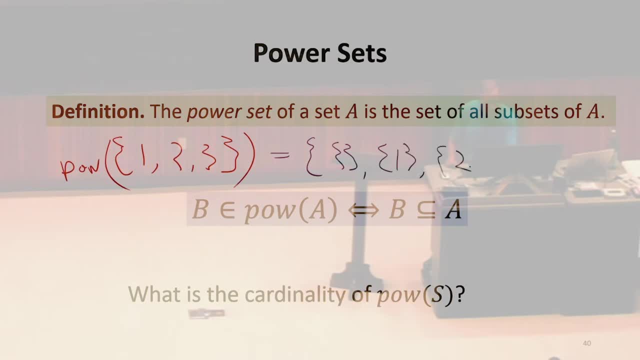 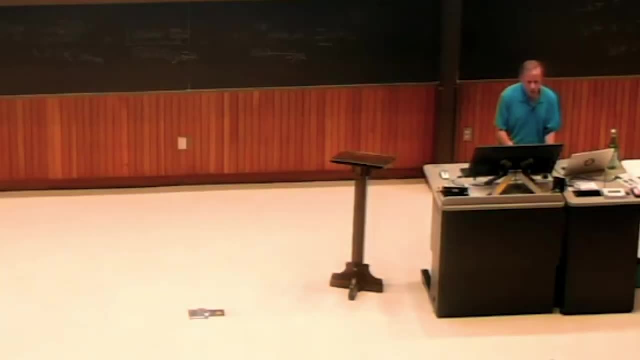 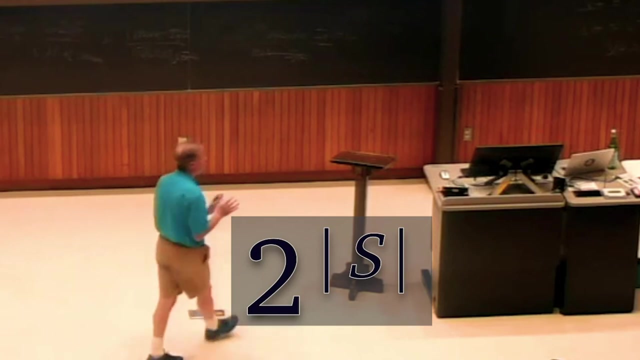 It's going to have the set containing 1, the set containing 2, the set containing 3, the set containing 1, 2, and so on. What is the cardinality of the power set? Yeah, good, How do we know this? Can we prove the cardinality of the power set? 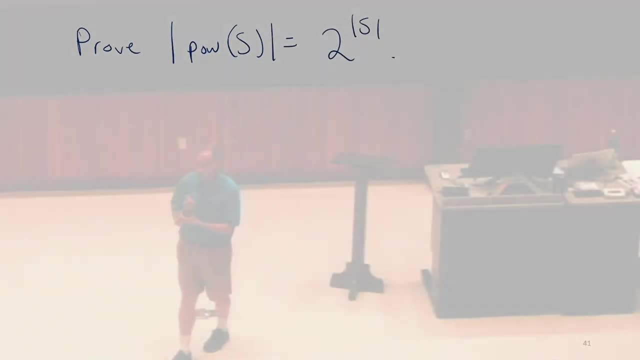 What strategy do you think we should use to prove this? Yeah, we can use our constructed definition of a set and we can say: either an element or the nth element that you're adding on there is in the power set or is either in the element. 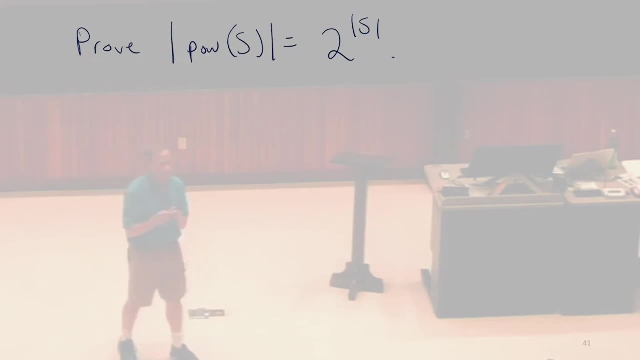 of the power set or it's not in the element of the power set, And that's two cases. It's going to be two times, whatever it means. Okay, good, That sounds on the right track. So as we add a new, 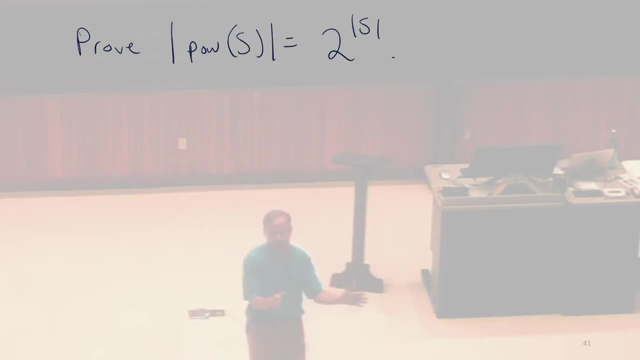 element to a set. the power set is the old power set plus the old power set, with that element added to every set. Can we be more clear how we're going to prove it? Yeah, did you have a question? Oh, I was just thinking about taking that and putting it into binary form. 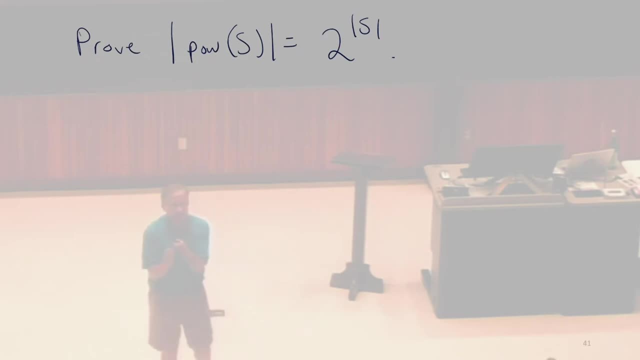 representing it as a binary string. Okay, yeah, that's actually a very clever idea. One way to think of the power set is a binary string where for each element in the set it's zero or one, whether that element is in there. We won't get today, but that's actually. 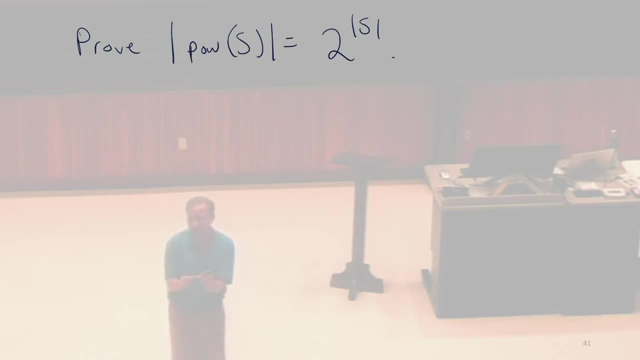 one way to see about the cardinalities is a very interesting way of looking at things. Yeah, You do it by induction with a base case and then for each step up you take every single element of that set and then you kind of just insert it into every one of those sets and then 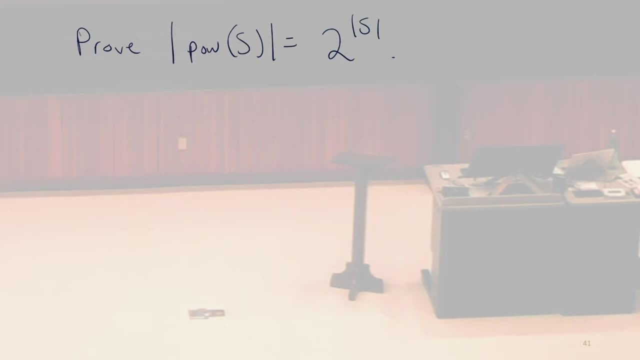 two of those together are the power set. Cool, okay, good, yeah, So this seems like something we can prove by induction. Proving by induction seems like a good strategy for this. Our principle of induction works on the natural numbers. We're trying to prove something about sets, Remember. 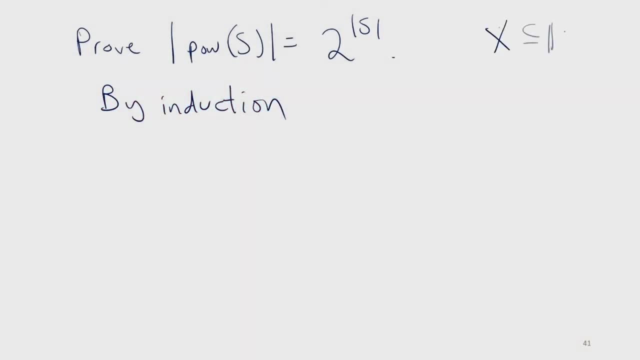 our principle of induction was: we're proving something about some subset of the natural numbers. We don't have a principle of induction for sets, yet What is the set of the natural going to allow us to prove something about all sets? The idea that she had is: you know, we 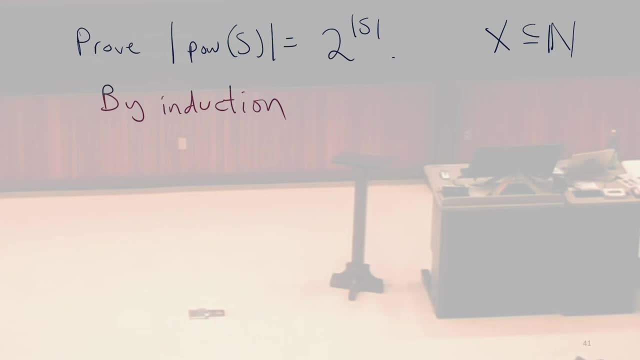 should prove this by induction right. Our intuition is that as we add elements, it's going to grow. This seems like a property that we can prove by induction. The problem is our principle of induction. what we've proven so far about induction only allows us to cover the natural. 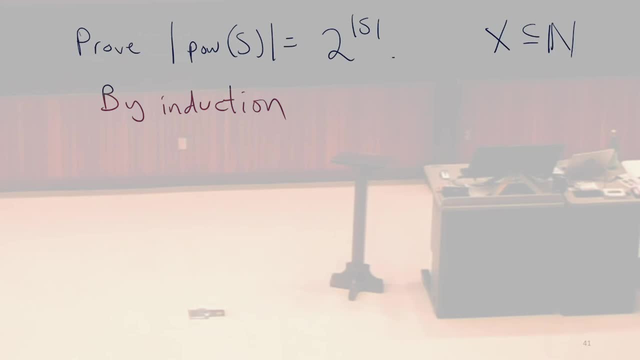 numbers. If we were trying to prove something about all the natural numbers, we've got our principle of induction. If we had that intuition of, yeah, we can show that as we grow the set this property holds, we would be there. But we're not trying to prove something about the natural 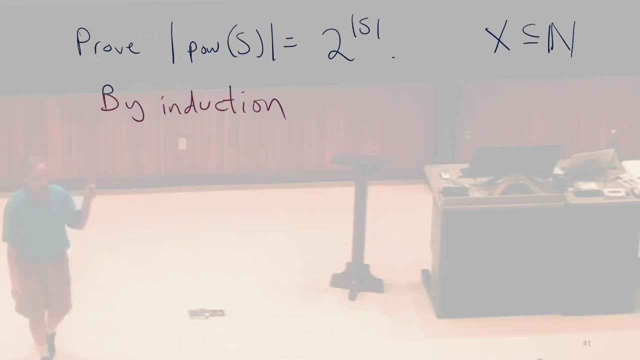 numbers. At least, we haven't stated it as a property of the natural numbers, We've stated it as a property of all sets. So what do we need to do to make this work? Did you have an idea? You have to limit this proof to countable sets. 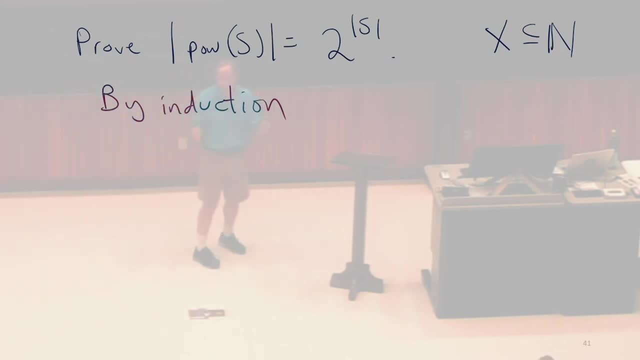 That's a very good point. Yeah, Our induction principle works for the natural numbers. We're only ever going to prove things about countable sets using it. This is only going to work for finite sets, But the sets that we're proving it on. this is we want to prove it for. 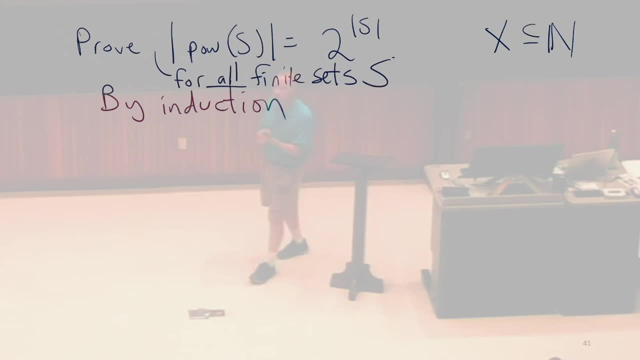 all finite sets, Because the finite sets are countable. in this case, these are sets where the elements don't matter. All that matters is how many elements there are, And certainly this property, when we're talking about cardinalities. the actual elements in the set shouldn't matter. 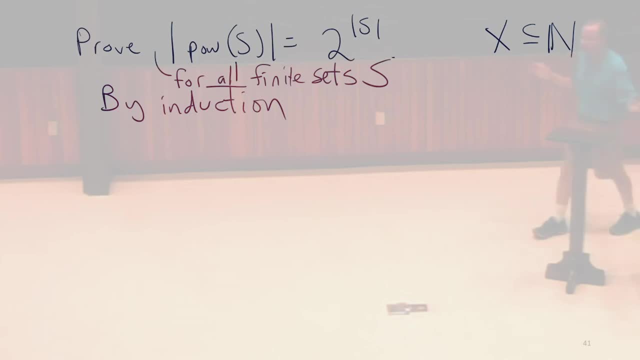 Right, So that's countable. And it's countable because the size of the set is all that matters, Right? And what are the size of the sets that we care about? if we're talking about finite sets, They're exactly the natural numbers. So we're going to be doing this induction on the cardinality.